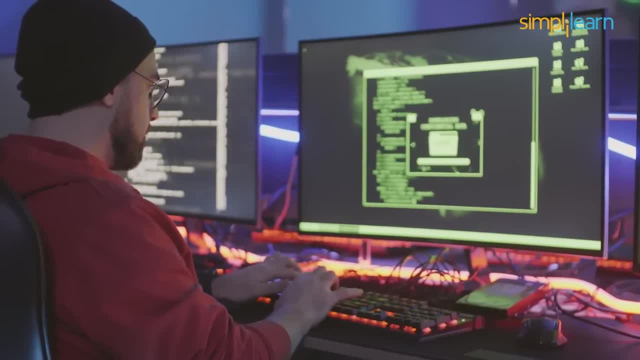 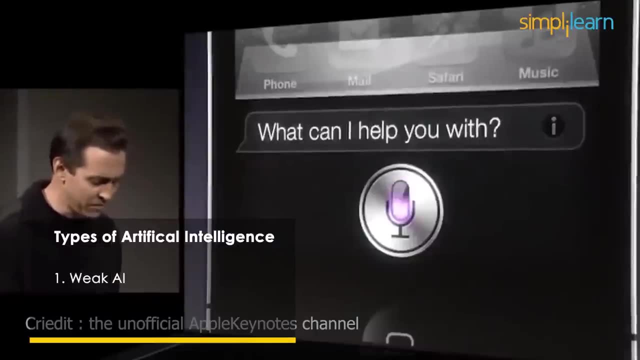 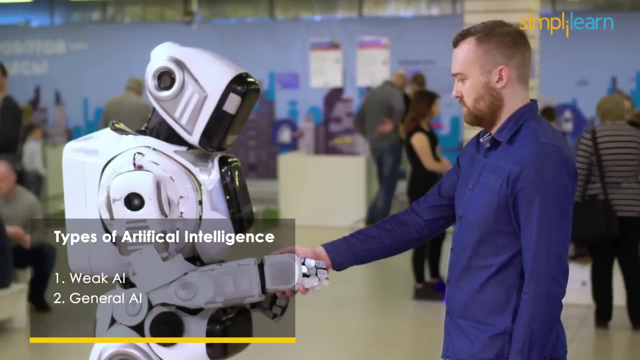 certain occupations, it still creates more jobs for humans. AI can be categorized into three types. Firstly, weak AI performs specific tasks, like Apple's Siri. General AI performs tasks like a human. The super AI is more capable than a human, but both are not as capable as a human. 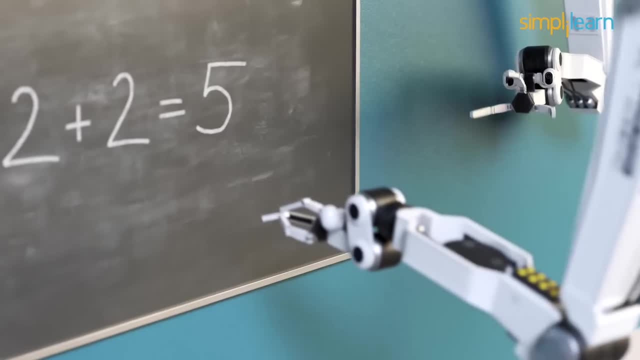 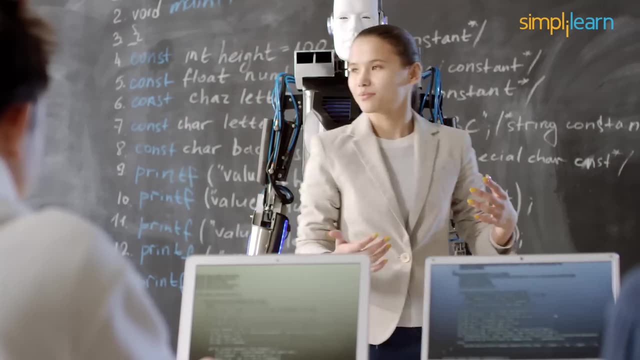 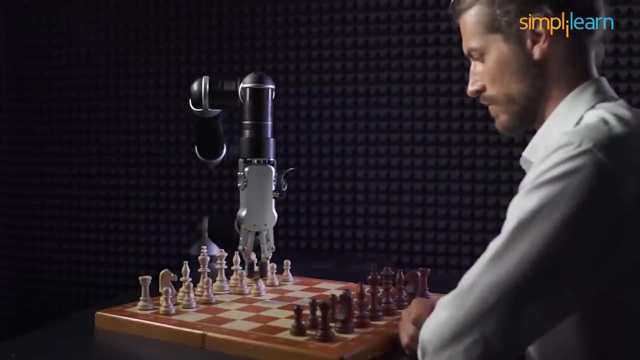 General AI and super AI are hypothetical because these technologies are not yet developed and research is ongoing. However, the development of such AI will take a lot of time. The development of AGI will accelerate within the following ten years. In fact, according to researchers. 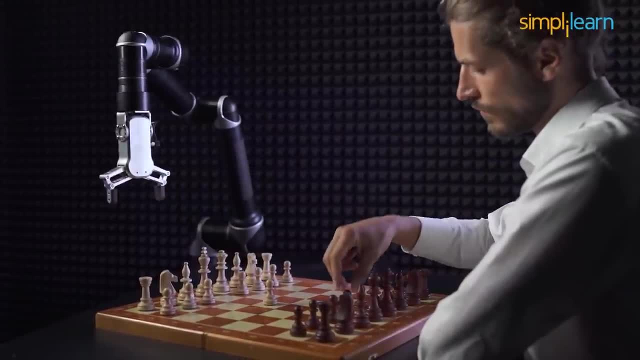 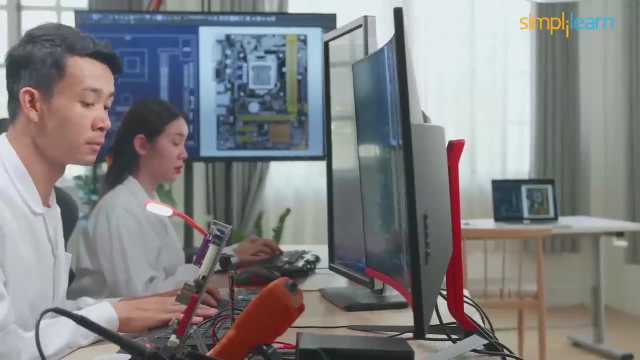 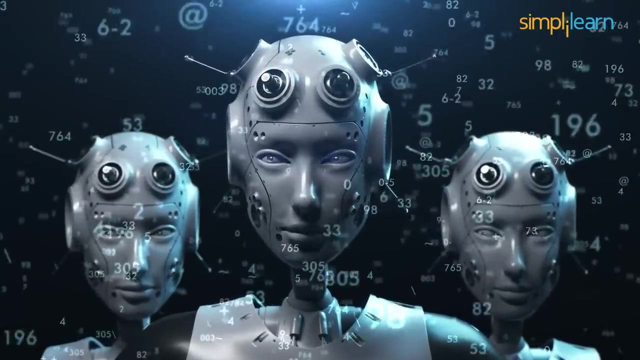 there is a 25% probability that by 2023, AI will resemble humans when it comes to thinking capacity. Additionally, the current data boom, computer development and computer developments, and improvements in automated methods and machine algorithms will provide a solid foundation for platforms with human-level AI. 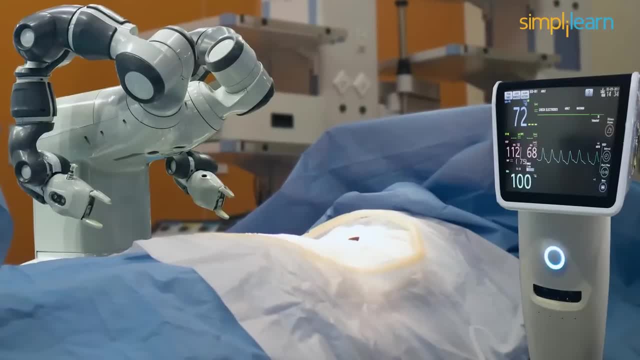 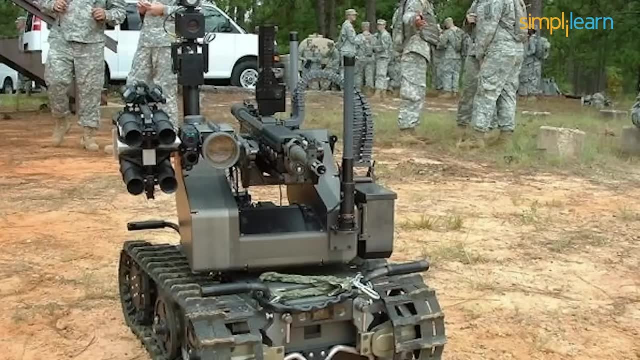 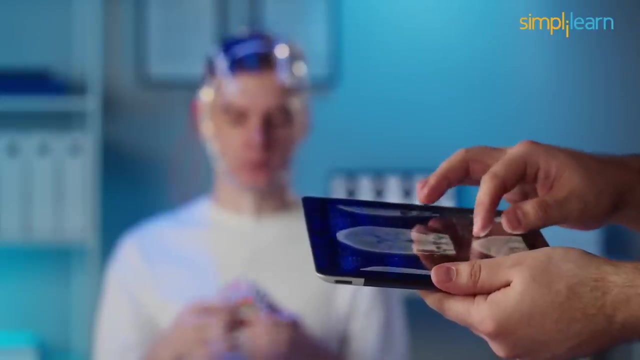 AI has occupied crucial sectors like healthcare, cybersecurity, e-commerce, agriculture, robotics, education, the military system, finance, gaming and many more. AI is used in healthcare to identify diseases, helping healthcare service providers and their patients make better treatment and lifestyle decisions. 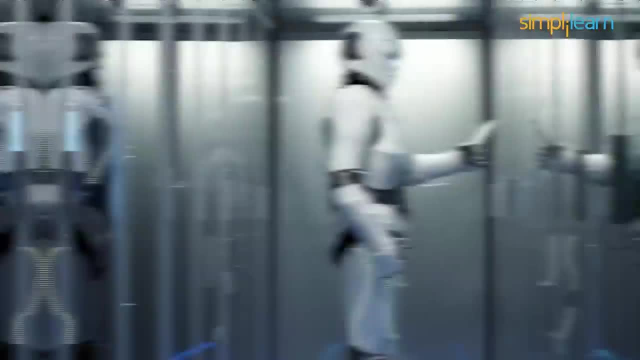 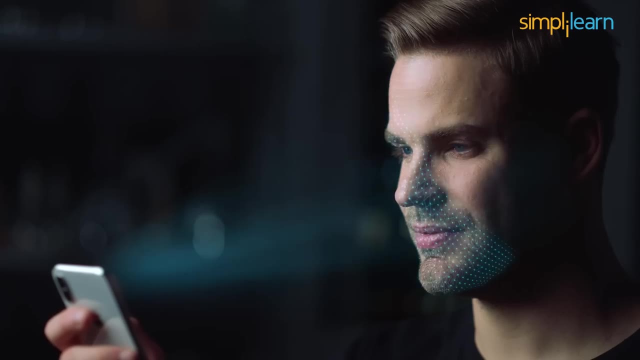 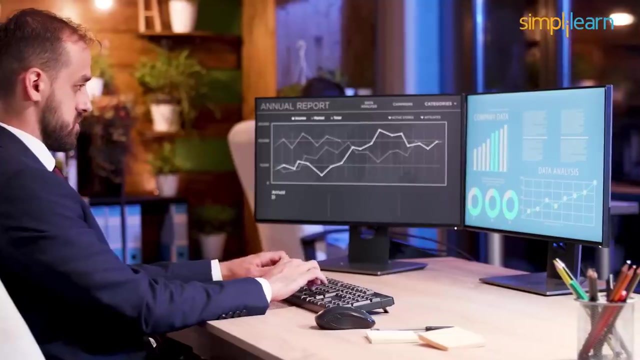 We can say that without AI, we couldn't have made the incredible recent advancements in fields like robotics, virtual reality chatbots, face recognition and autonomous vehicles. Smart robot advisors in finance, insurance, legal media and journalism will deliver instantaneous research or discoveries. 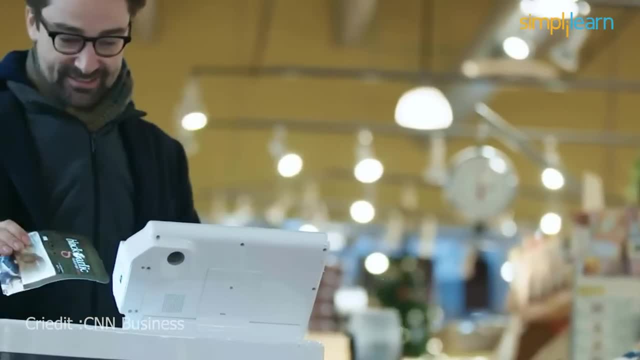 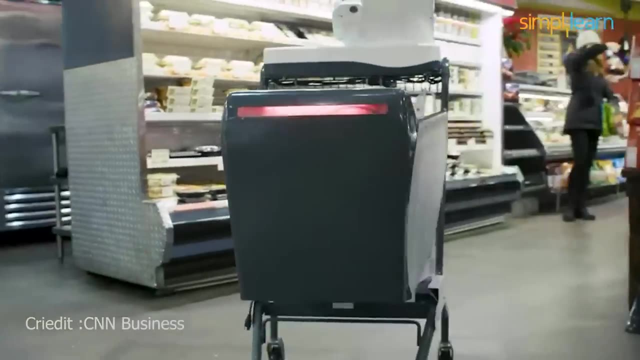 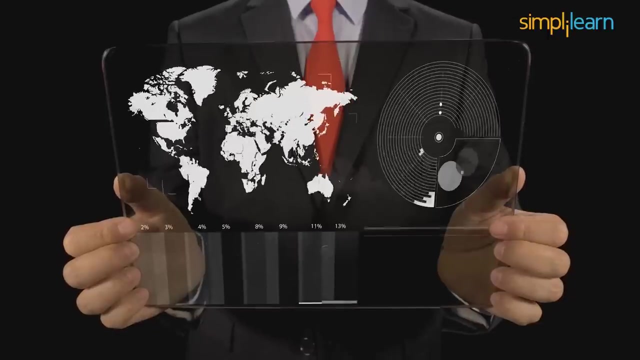 In the upcoming years, it is anticipated that artificial intelligence and machine learning will become more prominent in the consumer market, which will immediately affect how well web development functions. Virtual assistants or chatbots will provide professional advice. Other advantages include strengthening governance through better decision-making processes. 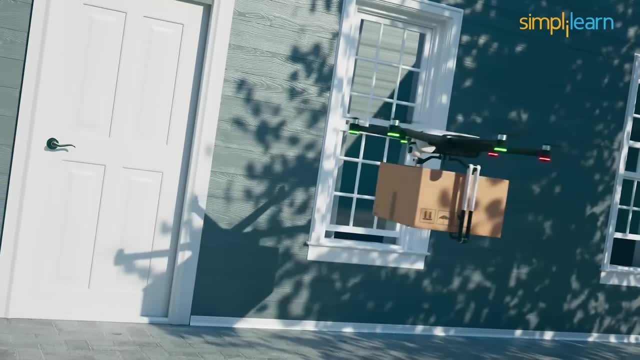 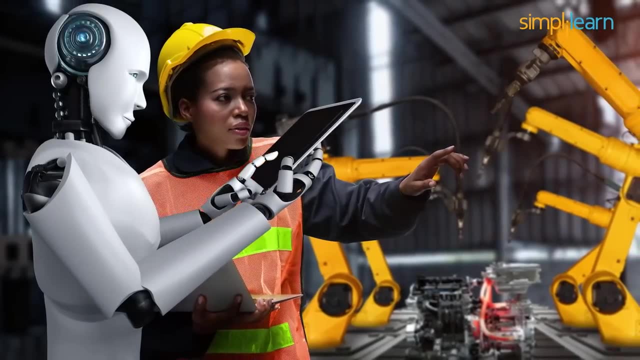 shortening time to market for R&D initiatives. and streamlining transportation and supply chain networks. Given all these scenarios, AI is all set to revolutionize, and to revolutionize every sector in the near future, Given that it is expected to impact 60% of firms.